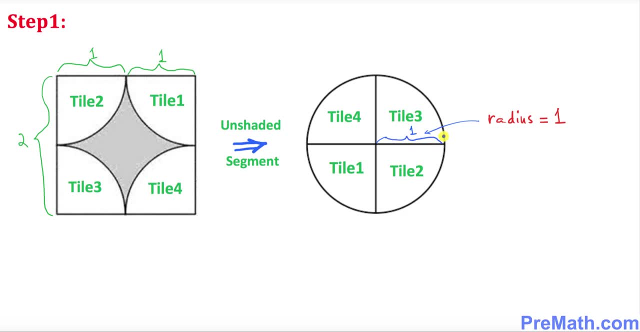 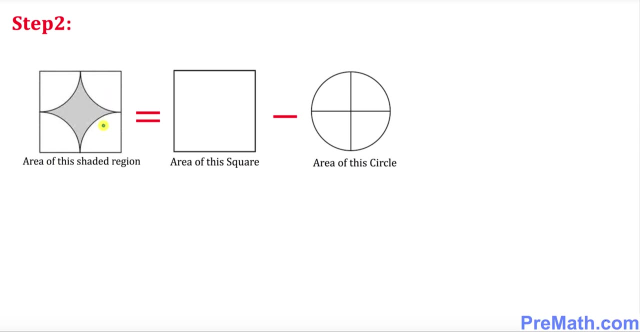 easily see that this radius turns out to be one unit. just this is the here. the simple formula will be using: the area of this shaded region equals to the area of this whole square minus the area of this circle, isn't it? because if you take away these circles, we ended up with just a shaded 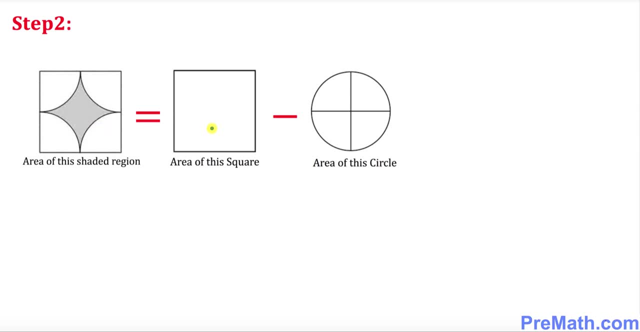 circle region. now our next job is going to be find the area of this square and this circle, and we will be pretty much done. and now we're going to find the area of this square. this the formula, where area is simply equal to the square of this side s, since each side is same. so in our case, our area. 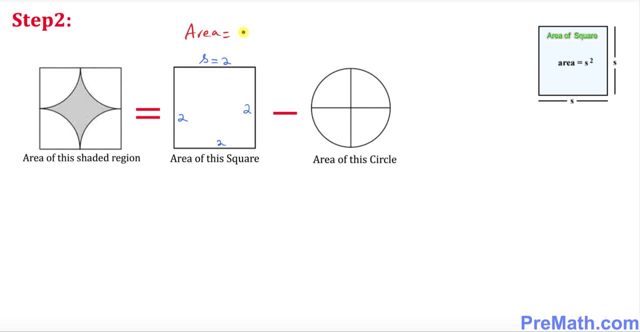 is going to be simply equal to two square, isn't it? because s is two, which turns out to be four. so our area turns out to be four of this square. and now to find the area of a circle. here is the area of a circle. formula a equals to pi r. 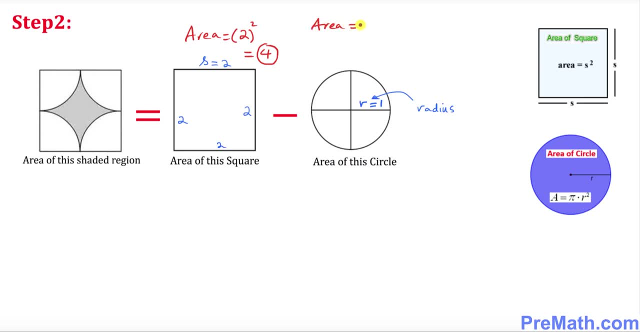 square. so you put down area equal to pi r square and we know r equals to one unit, so that's going to be a pi times r is one square, so pi times one, equal to, just simply, area turns out to be pi. so far, so good, and now let's go ahead and take care of this thing. so the area of this. 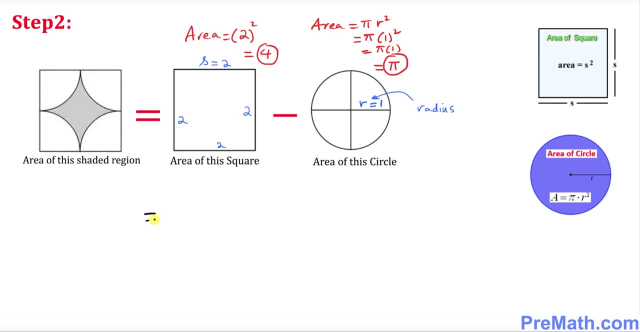 shaded region is going to be equals to this area turns out to be four minus the area of this turns out to be pi. if you want to leave your answer in terms, this one, that is your answer. and if you want to find the value of pi, and the value of pi is 3.14- we know that thing, so let's go ahead and put down.